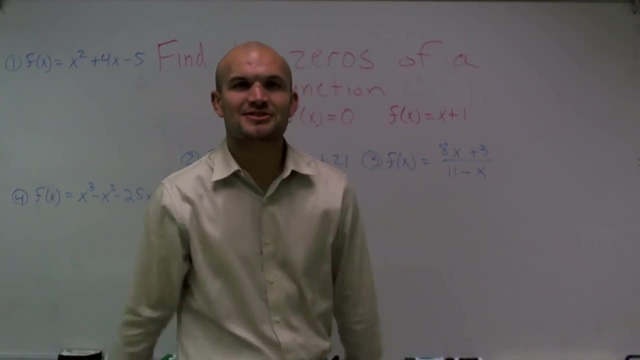 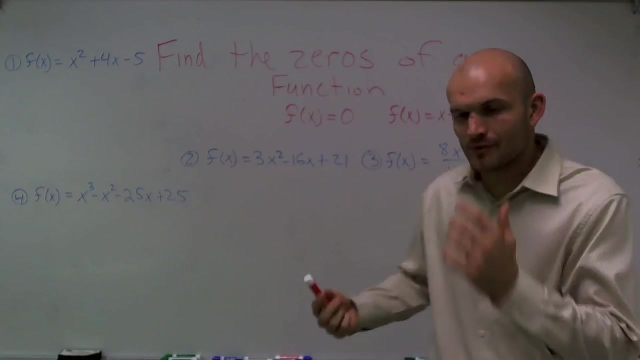 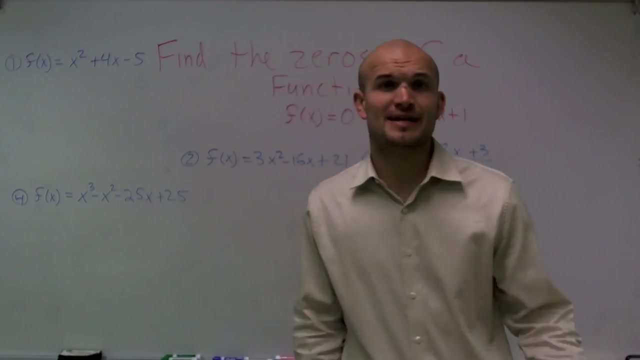 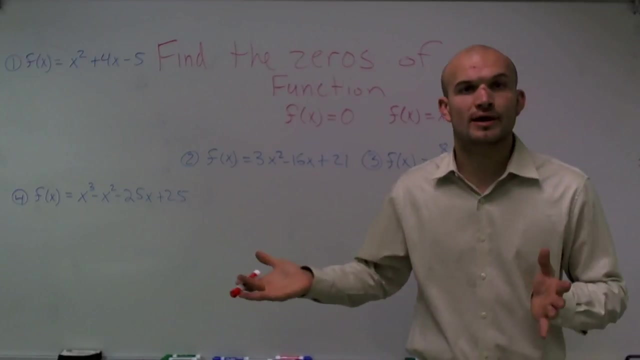 Welcome. What I want to do is show you how to find the zeros of a function. So, when finding the zeros of a function, what we want to do is really understand what are zeros and why we try to find them. Well, there's a couple explanations. There's a lot of different definitions for zeros, But the main important thing, if you can think about it, remember a function: we have our input and our output right. 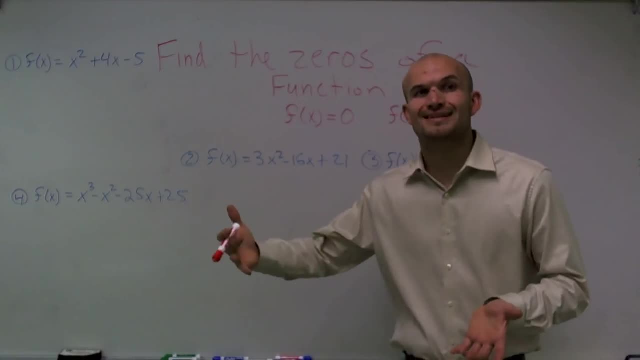 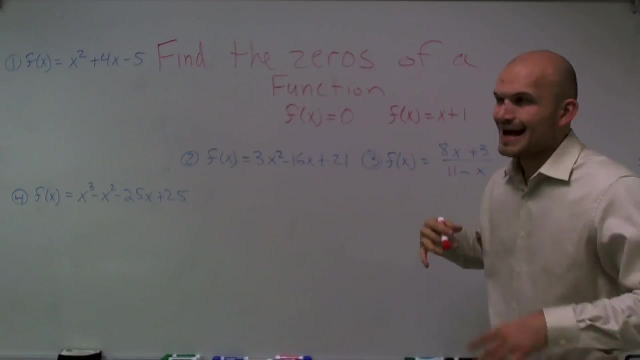 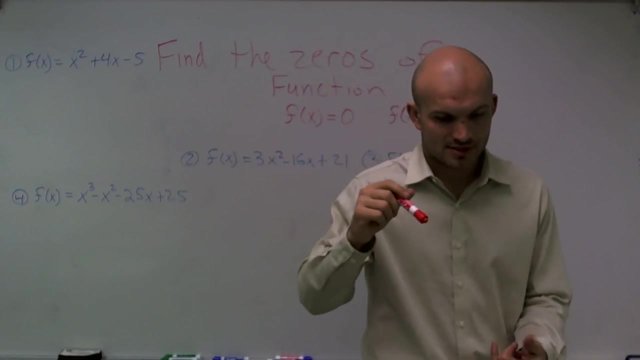 Well, the zeros of our function is when our output is equal to zero. So what we say is f of x, which is our output equals zero. So any x value that I input where it gives me an output of zero is what we call a zero. And you know the zeros are very helpful for us because you know those are actually the x-intercepts of a graph of any kind of polynomial that you're working with. 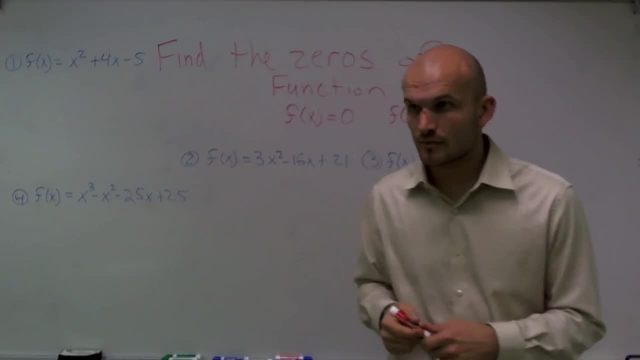 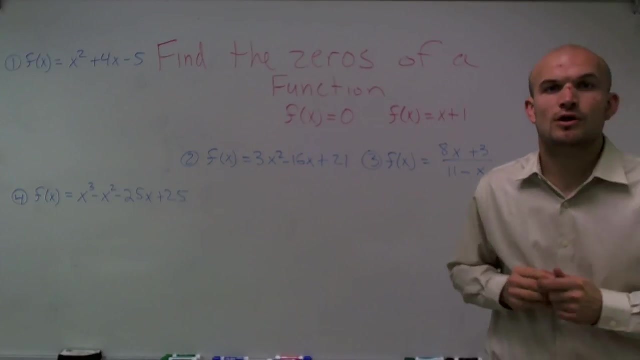 And you also call them sometimes. you know your roots. So let's look at something very basic and I'll kind of show you how we're going to find our zeros. So the first one is: let's say I gave you a function, f of x equals x plus one, And I say: find the zeros of that function. Well, what that means is I want you to find what are the x values that I have to plug into this function to get my output equal to zero. 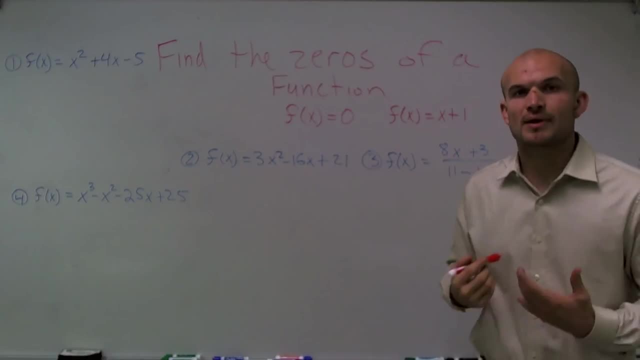 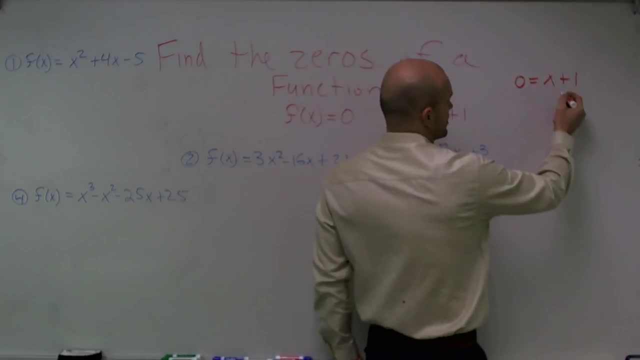 Now for this problem. we can probably do it in our head, But it might be helpful for us to write it out as an expression or an equation. So zero f of x equals zero. Zero equals x plus one. Now to find the value of x that's going to make that equal to one or zero, I just subtract my one on both sides and I get negative. one equals x. 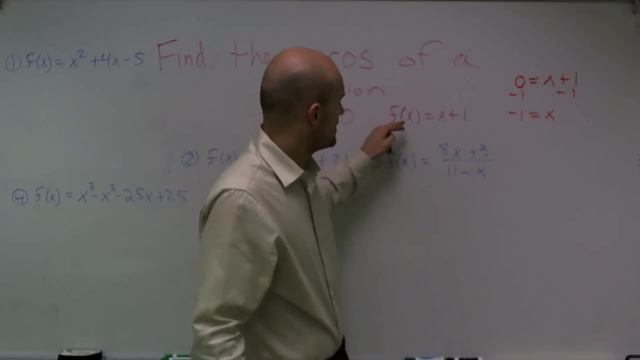 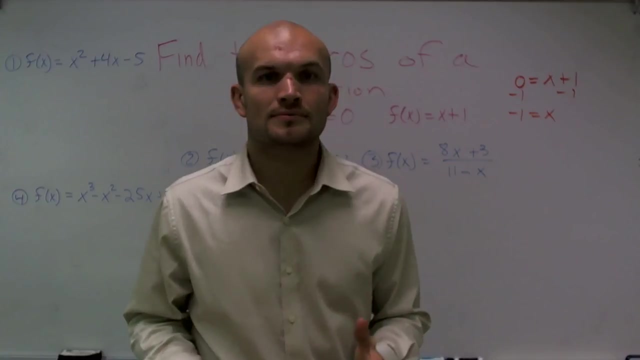 So what that means is, whenever I plug in a negative one for my x, my output is equal to zero, which we know is true. Negative one plus one equals zero. Now this gets a little complicated now, because what we're going to be doing is we're not just going to be dealing with linear functions. 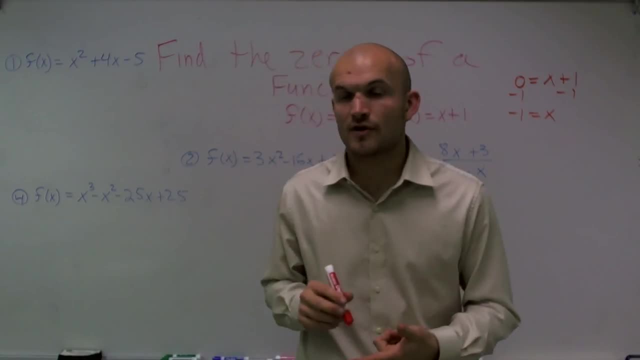 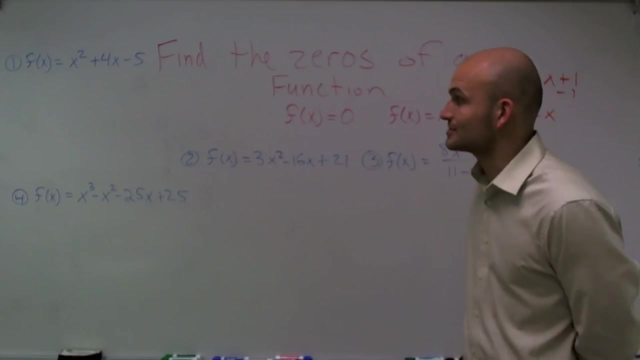 We're going to start dealing with quadratics, Quadratic functions and functions to the third and fourth degree. So it's going to get a little crazy and we're going to talk about rational functions. But if we can just keep the same idea in mind when we're trying to find the zeros, we need to set it equal to zero, set your output equal to zero and then find the values of x. 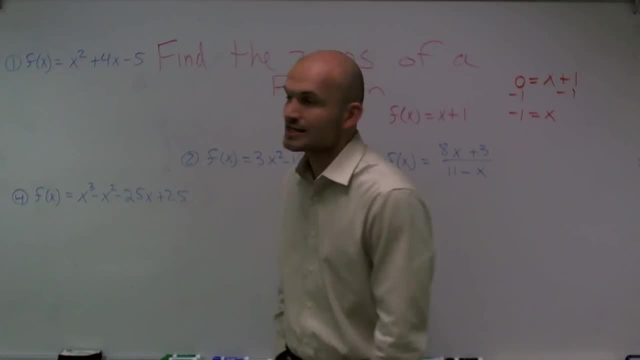 So let's look at question number one. It says f of x equals x squared plus 4x minus 5.. So I plug in a zero for my f of x. I have zero equals x squared plus 4x minus 5.. 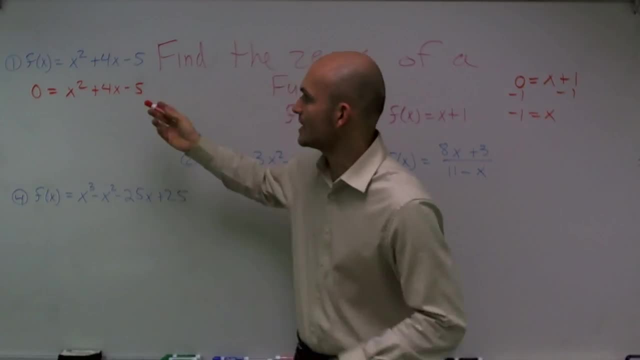 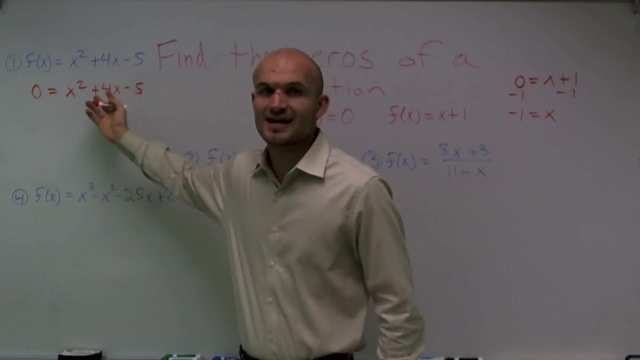 Now, a big problem that a lot of students want to do is they just want to solve for x. They want to put the 5 over there, put the 4 over there, square root it all this kind of stuff. Well, one thing we need to know, ladies and gentlemen, is when we have a quadratic, it's very difficult when we have two different x's. 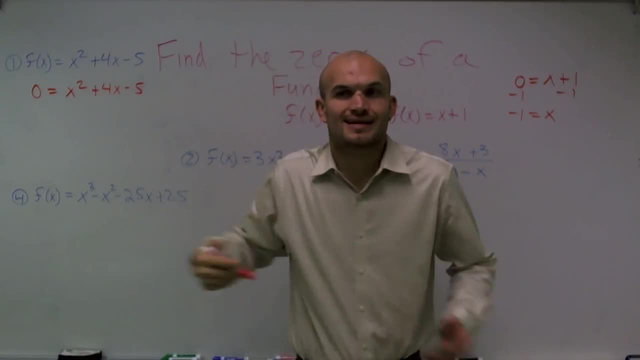 We have an x squared and an x that we can just solve. for the x, We're not going to be able to do it, But for us to solve this, what we're going to have to do is we're going to have to. 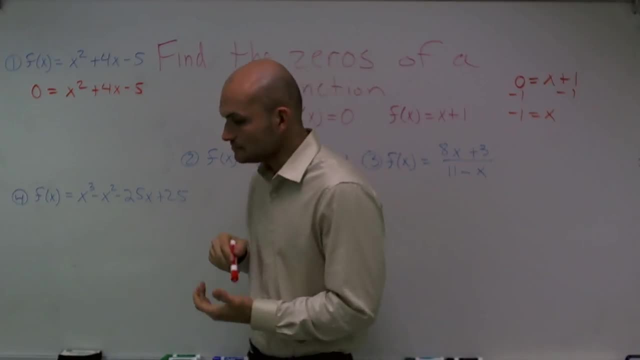 Factor it. So we're going to have to look at our factoring And so to factor this, whenever we have our a is equal to 1,. what I can do is set up a- you know, a diamond method per se. 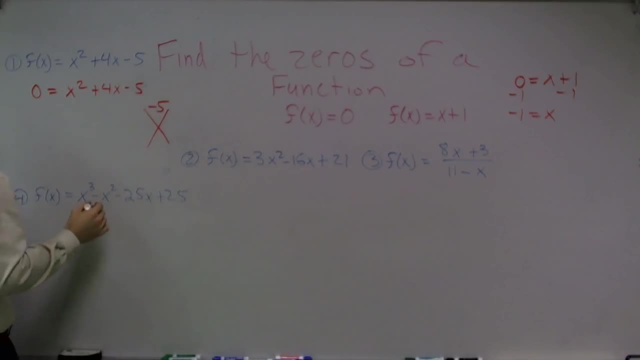 And what I can say is I take my last number, negative 5,, which is my constant, and I take my middle number, which is 4.. And I say: what two numbers multiply to give me negative 5, but add to give me negative 4?? 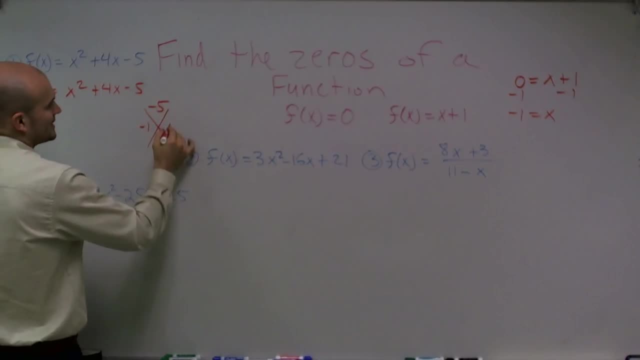 And I can say: well, negative 1 and 5.. Negative 1 times 5 gives me negative 5. But negative 1. Plus 5 is going to give me 4.. So what I can do now is I can write this, as we're going to call two factors: 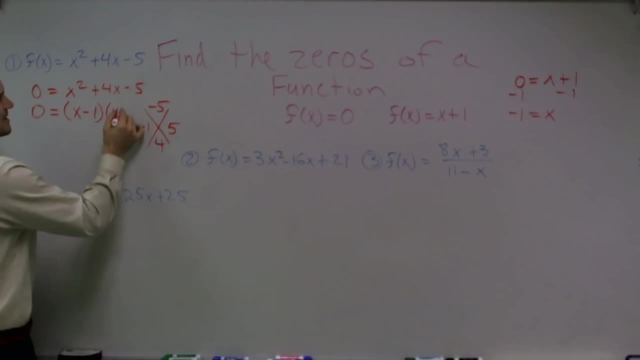 x minus 1 times x plus 5.. And if we were to foil this out by multiplying by using your foil method, you would get exactly this quadratic again. Well, one thing we notice is whenever one factor times another factor equals 0, one of them, what we say, is going to equal 0. 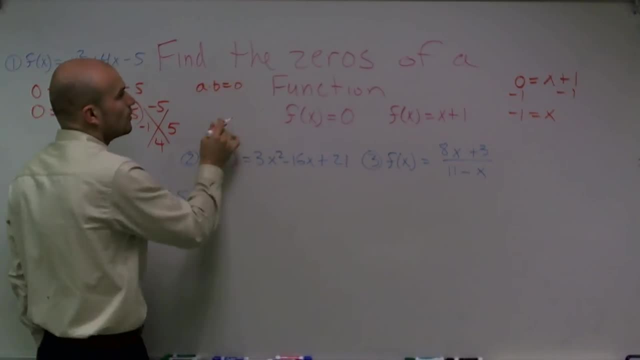 Okay, Just like if I say a times b equals 0, one of these has to equal 0. So what I do is I set both of these equal to 0. I say x minus 1 equals 0 and x plus 5 equals 0. 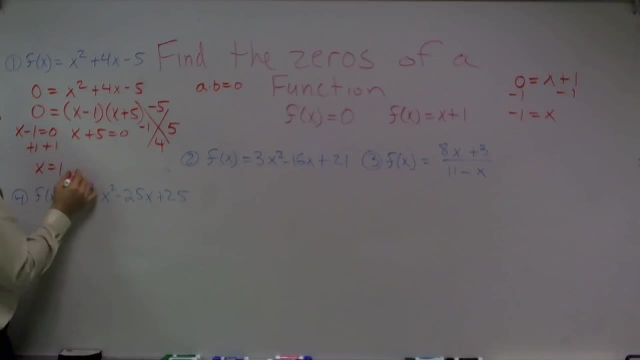 Now solving for x, I get x equals 1 and x equals negative 5.. Therefore now the 0s for this equation are positive 1 and negative 5.. Now let's move on to number 2.. Number 2 looks like it's a little bit more difficult problem because now I have an, a, my number in front of my x squared is not 1.. 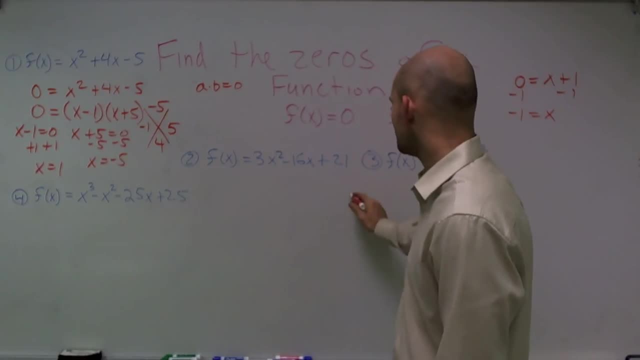 So it's going to be a little bit difficult. I can still use the diamond problem, But now when I use the diamond problem I need to multiply my 3 times my 1.. So 3 times 1 is going to give me 63.. 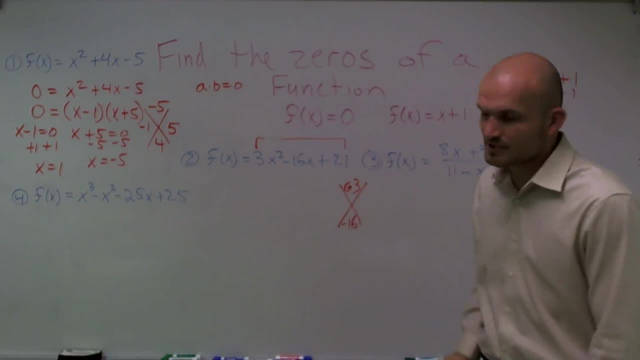 And then I have a negative 16.. So what? two numbers? multiply to give me 63, but add to give me a negative 16? Well, our two numbers, Our two numbers are going to be a negative 9 and a negative 7.. 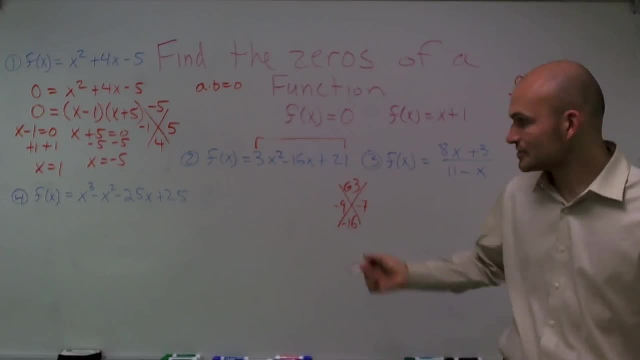 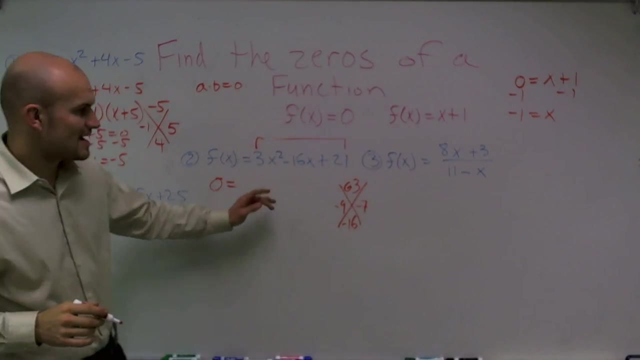 Now to write this as my factors, remember, I need to plug 0 in for f of x, So I'm going to say 0 equals And instead of writing the factors, I don't know what the factors are. A lot of students want to say: oh, it's x minus 9 and x minus 9 times x minus 7.. 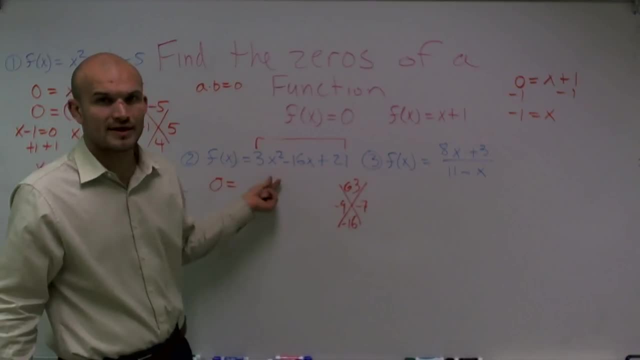 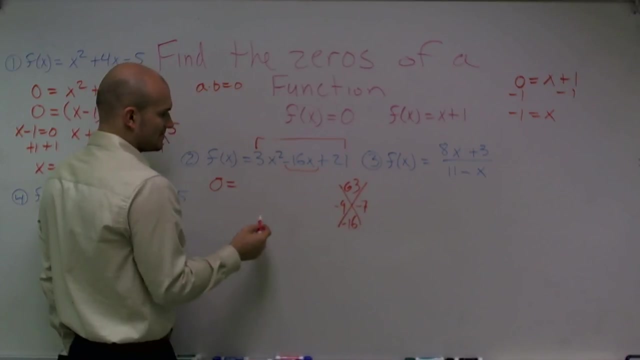 Well, if you multiply that out, that does not equal this. So what we're going to do is I'm going to rewrite my two factors In place of my negative 7.. So I'm going to say 3x squared minus 9x minus 7x plus 21.. 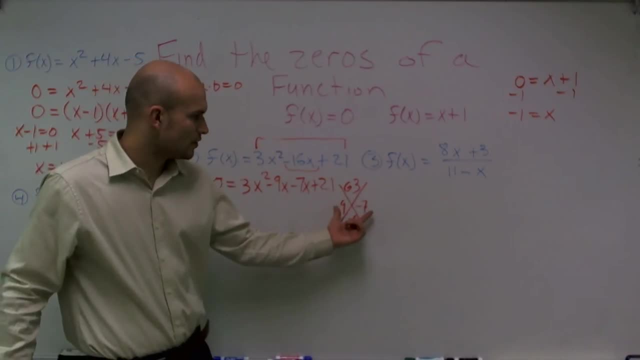 Now I can do this because what you guys can see is all I did is I rewrote these two numbers to add up to negative 16.. So I really these two add up to negative 16.. So I really didn't change it. 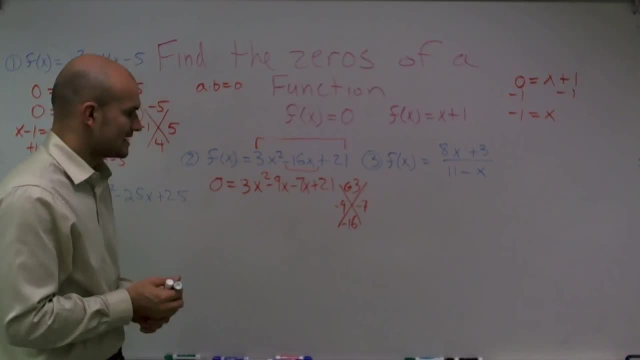 I just kind of rewrote it. Well then, what I can do is I can factor by grouping, So I'm going to group the first two terms and group the last two terms. Now I can factor by grouping So I can factor out my common term. so I have 0 equals. I can factor out a 3x. 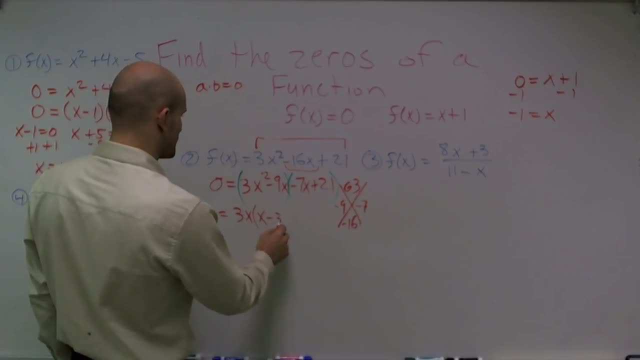 I'll be left with an x minus 3, and here I can factor out a negative 7, and I'll be left with x minus 3.. Then I can factor out a negative 3 or x minus 3,. so 0 equals x minus 3 times 3x minus 7.. 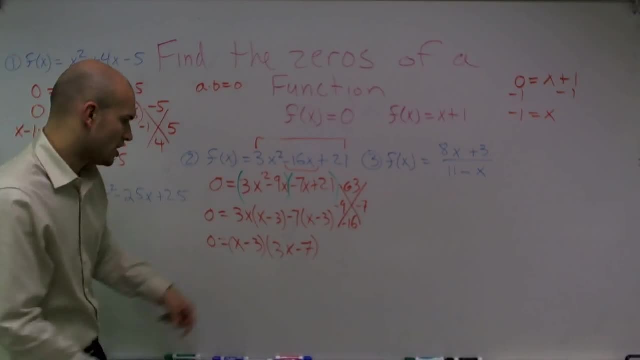 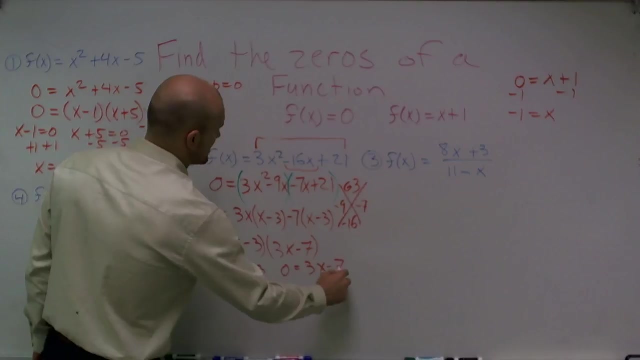 Now, doing like I did in my first problem, I'm going to solve each one of these and I'll have 0 equals x minus 3 and 0 equals 3x minus 7.. Now I simply solve: add 3 to both sides, x equals 3, and when I add 7 and then divide by 3,, 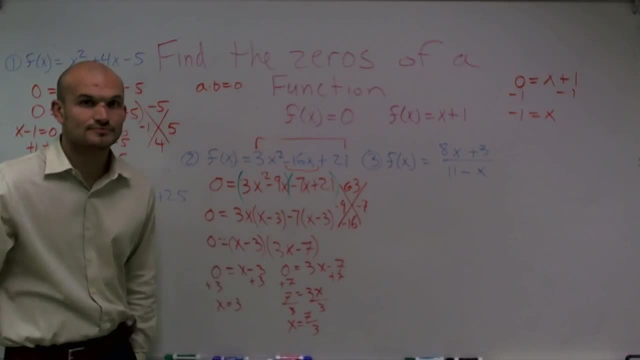 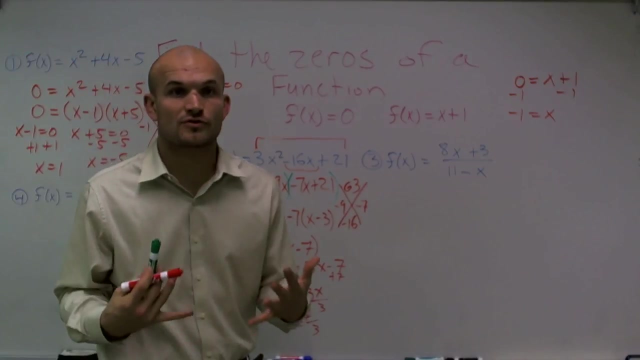 by 0 for this one is x equals 7 thirds. So that's how. that's a quick little review on factoring. You're really going to have to make sure, when you're finding zeros, that you're really good at your factoring. 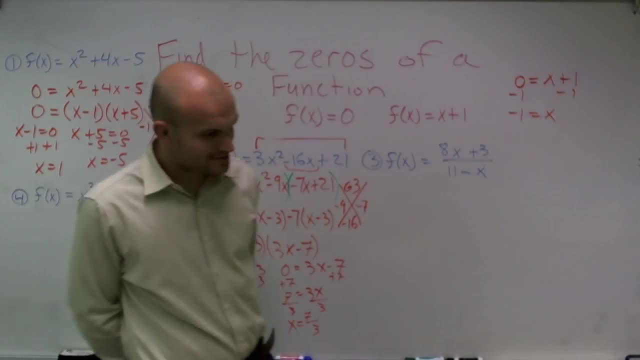 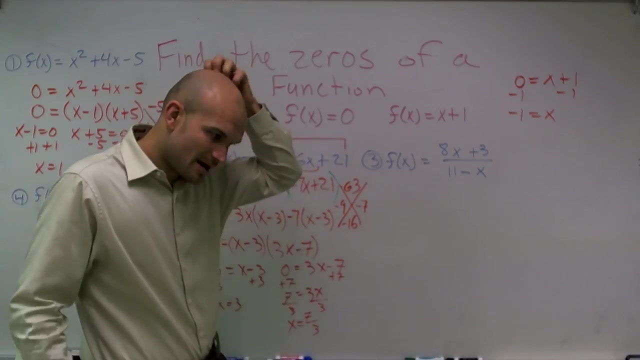 Number 3, this is what we call a rational function, and this one gets students all the time because they hate fractions. We hate fractions. Well, if we can remember first thing, who cares about the fraction? Let's just do what we know how to do, which is put a 0 for f of x. 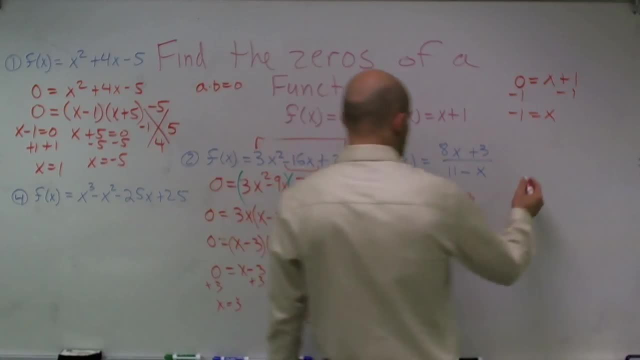 Now I'm going to go back to a simple problem here. and let's say I had 0 equals x over 7, or I don't know. let's put this as 2.. If I want to solve for x, right, I need to get rid of the 7,. what do I have to do? 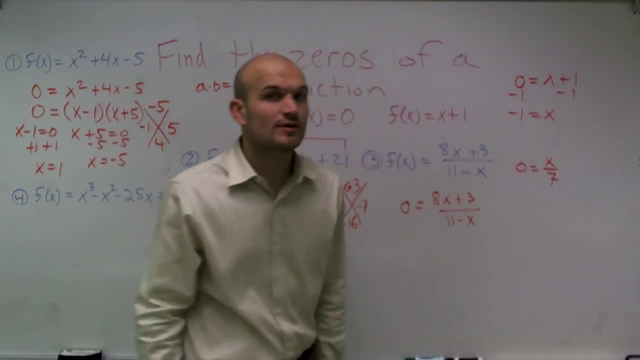 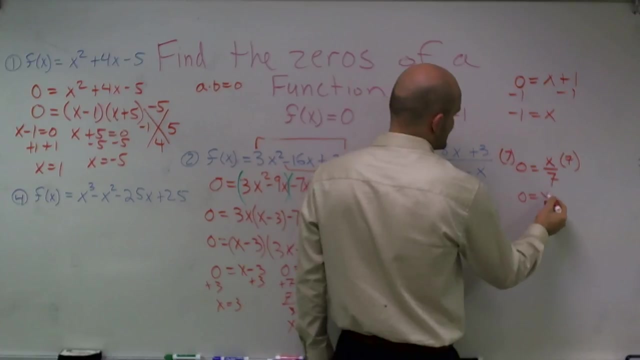 Actually. no, let's just put a 0 there. we'll help that. What do I have to do to get rid of that 7?? Well, I need to multiply by the 7, and therefore what you end up getting is x equals 0.. 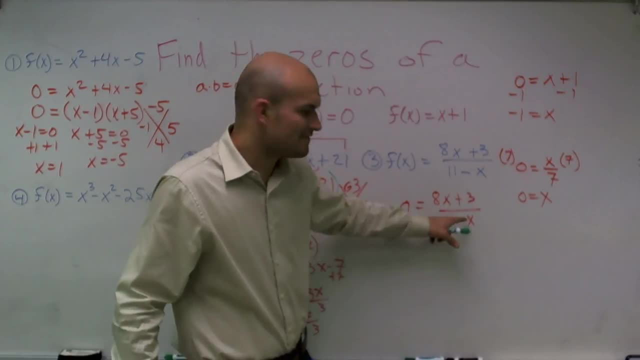 Well, this problem is no different. I have an 11 minus x on the bottom of my fraction, so to get rid of that, I need to multiply by the 7. So I'm going to multiply by 11 minus 7.. 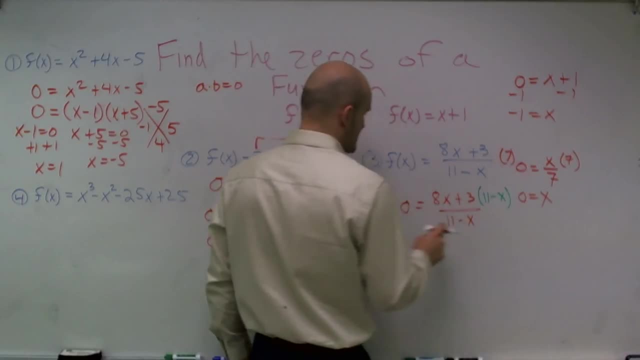 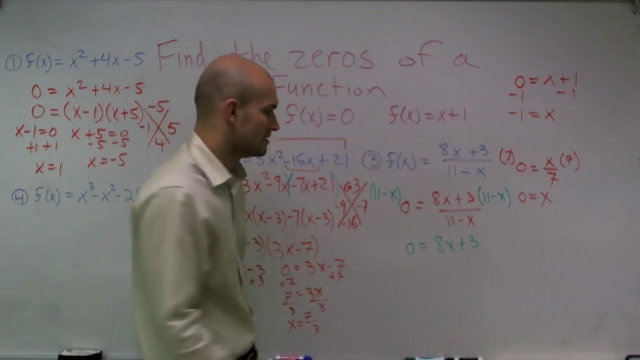 And what you'll notice is actually these problems are really really cool. because guess what? What is any number times 0? 0. So I end up getting 0 equals 8x plus 3.. And now it's very easy. this is just a, you know. now it's linear. 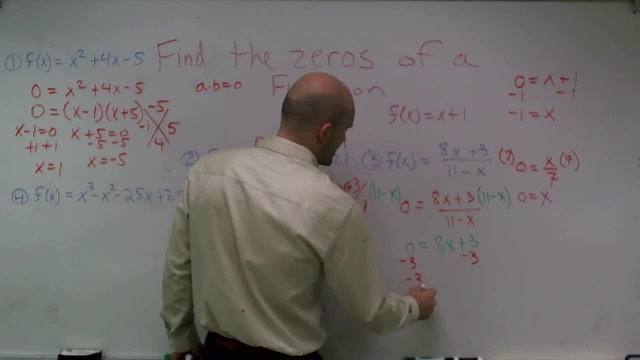 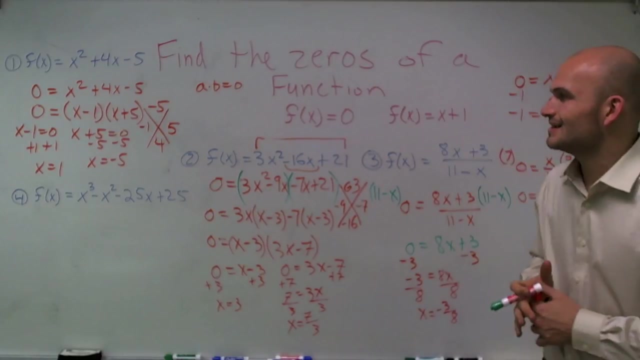 I can just solve subtract 3 on both sides. negative 3 equals 8x. divide by 8, x equals a negative 3x. All right, whew, one more to go, And this one's my favorite one, because nobody likes factoring by grouping. 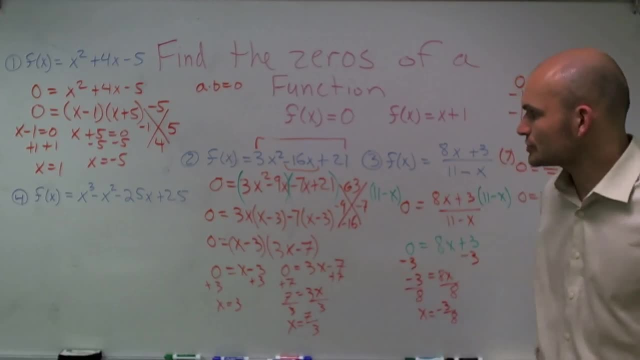 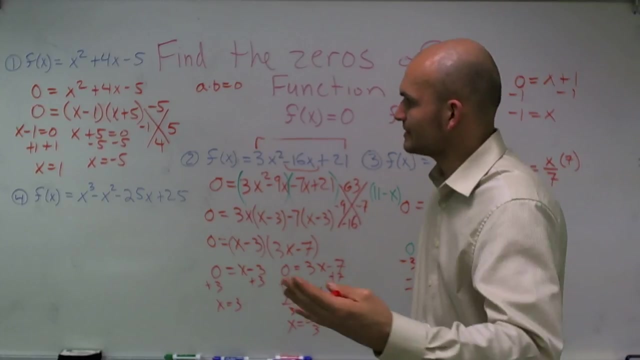 Factoring by grouping is actually what we did here, but it usually trips up a lot of students because they say, oh, four terms, crap, let me see if I can factor. or you know, I can't factor the same thing out. 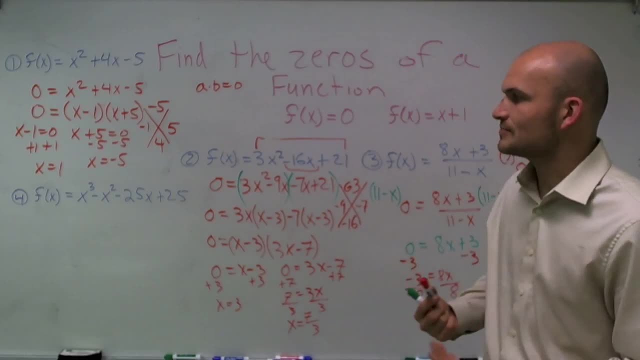 Remember, when you want to do factoring by grouping, the best way to do factoring by grouping is just to group your first two terms and group your last two terms. So, on my first two terms, what can I factor out? Well, I can factor out an x squared. 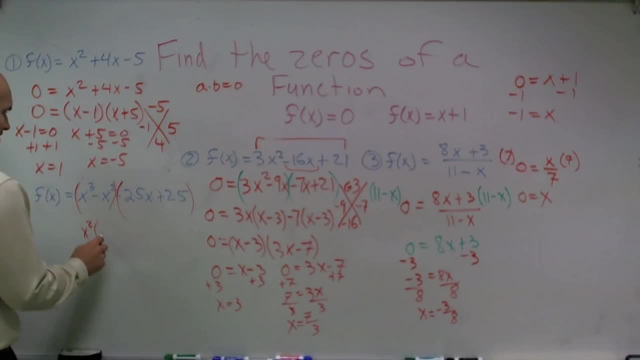 When I factor out an x squared, I'm left with x minus 1.. Then out of these last two terms, that's a negative 25, I can factor out a negative 25.. When I factor out a negative 25, I'm left with an x minus 1.. 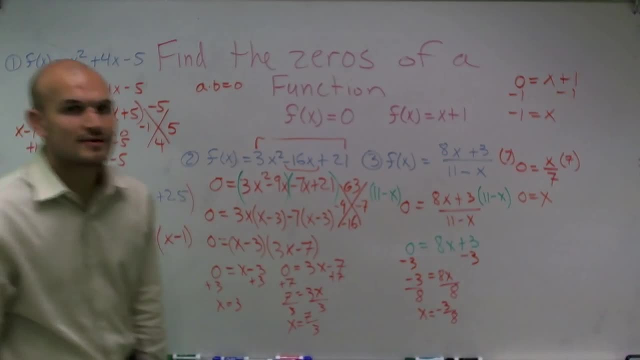 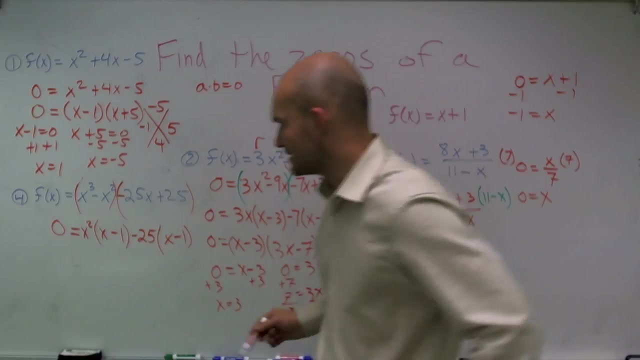 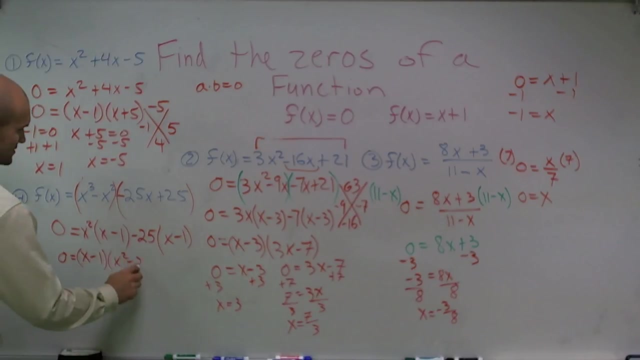 And I'm sorry I'm getting a little lazy- Remember that equals 0, right, Because f of x equals 0.. So now what I need to do is set these: factor out: an x minus 1, so I say 0 equals x minus 1 times x squared minus 25.. 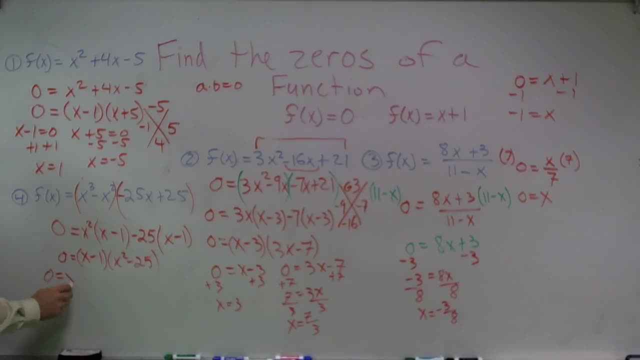 Okay, Now I set these both equal to 0,. 0 equals max minus 1, and 0 equals x squared minus 25.. So when I add 1,, I get x equals 1, and then here, just to kind of simplify it, I'm going to add 25.. 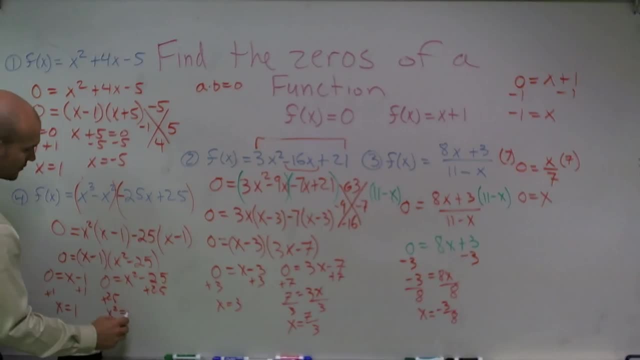 And then I'm going to have to take the root. so I have x squared equals 25.. Remember, when you take the square root, remember when you take the square root of both sides, you're going to get the positive and the negative of your root. 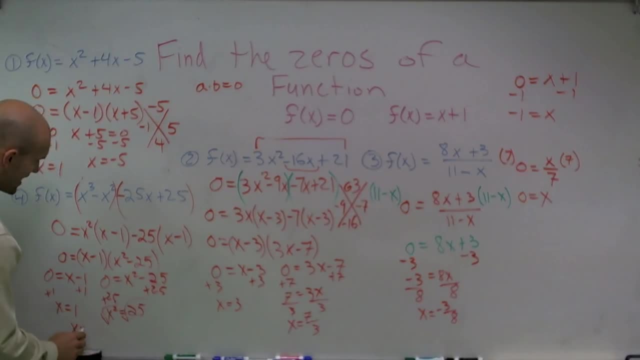 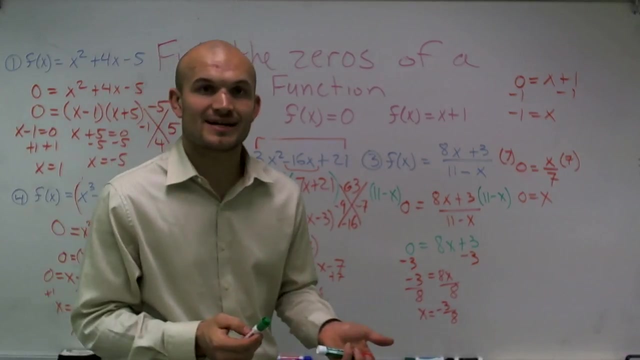 So, therefore, my zeros are going to be x equals 1,, x equals 5, and negative 5,, because 5 times 5 is 25, and negative 5 times negative 5 is 25.. All right, guys. 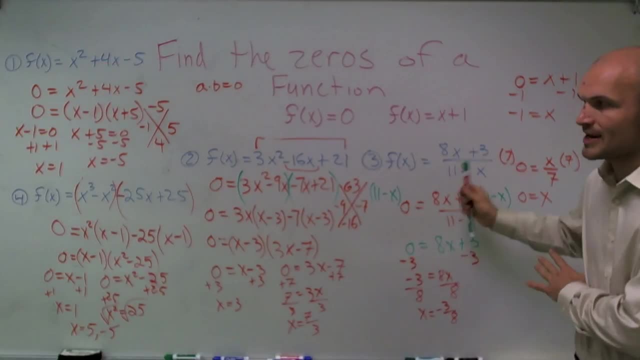 That's a lot of work I just put there on the board, So I'm going to leave that up there. I'm going to erase it here for a second. I'm going to put three problems up there that I want you to do. 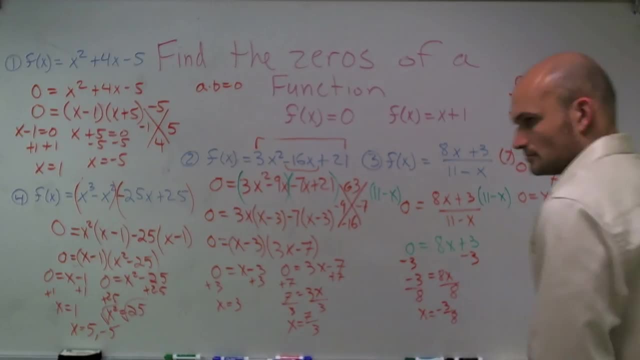 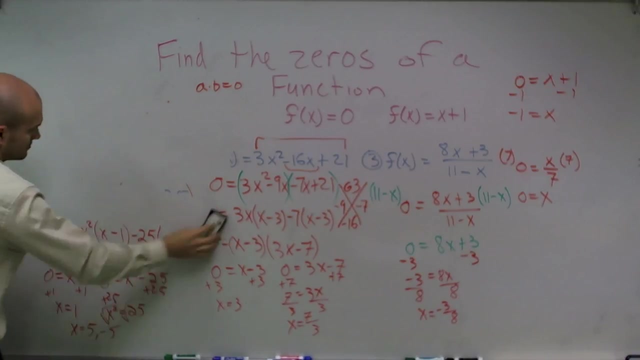 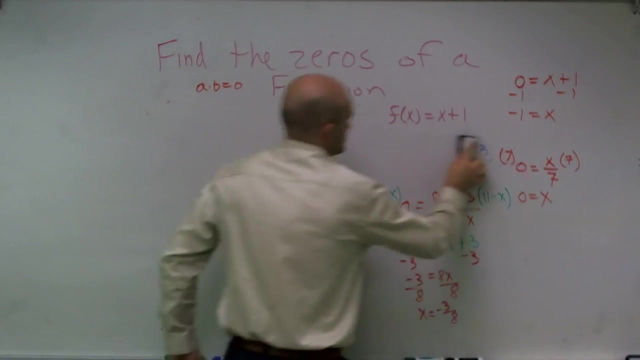 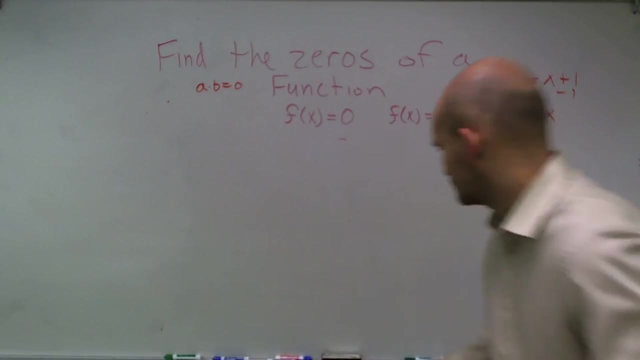 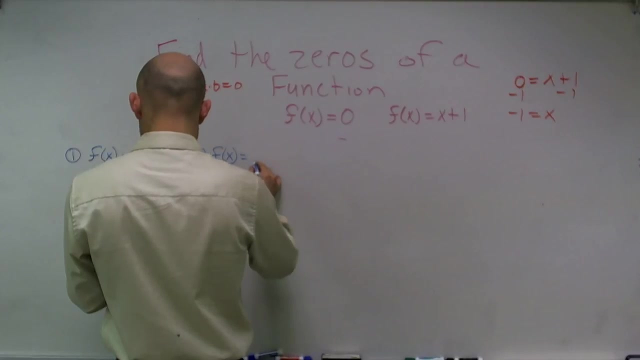 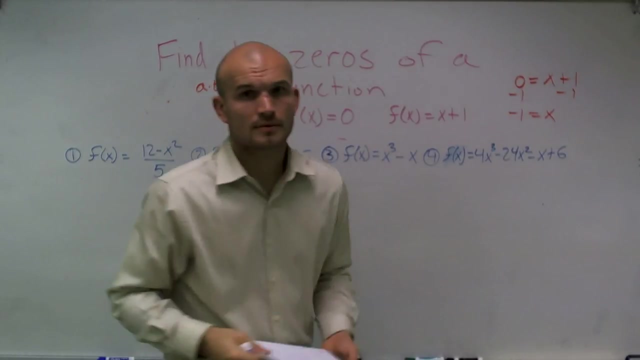 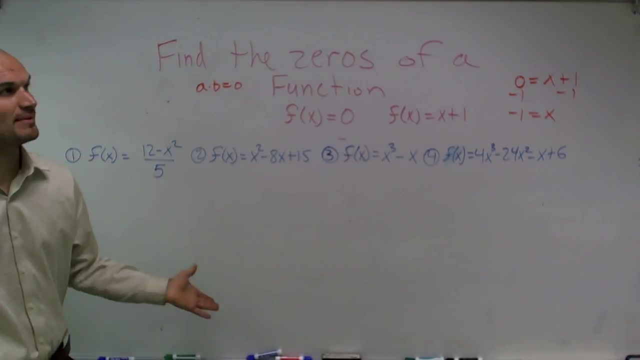 and then I'll show you the answers. All right, guys? Okay, What I'd like you guys to do is write down these four problems, give them a shot, spend about 5, 10 minutes on them, and then I'll come back and show you the answers. 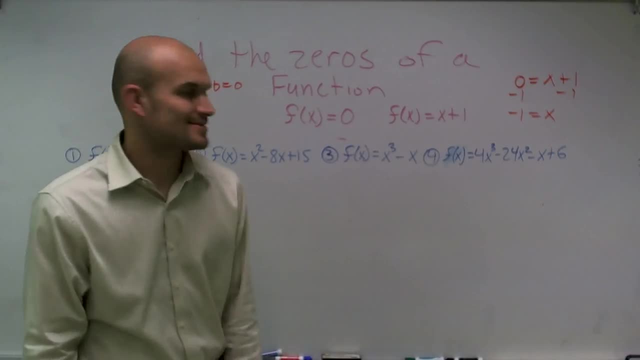 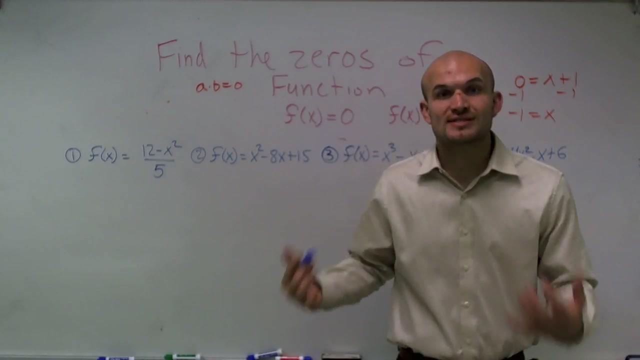 All right, You guys ready for this? Let's do it. First thing, guys, I'd like to do for all these problems, before you even start factoring, remember zeros- is when f of x equals 0.. So the first thing let's do is let's set f of x equal to 0. 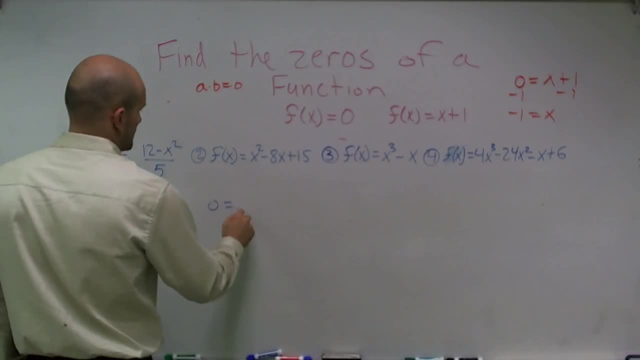 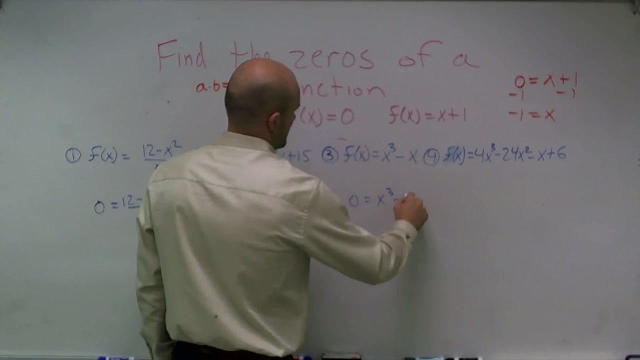 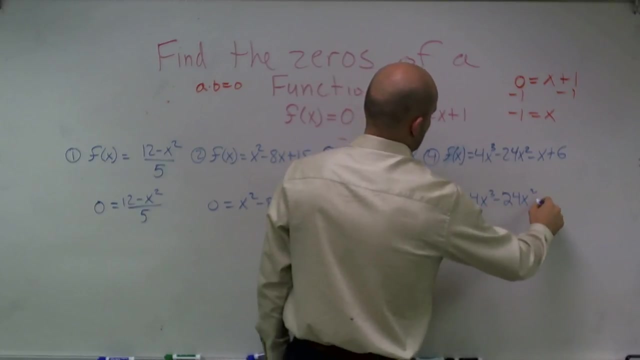 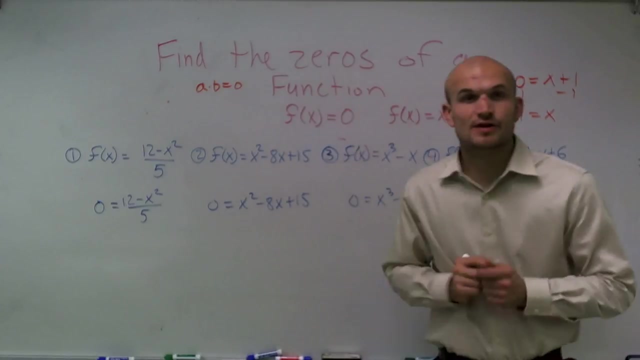 Okay, Now let's go back to the first problem. So the first problem is a rational expression or a rational function. Remember, when it's rational, we need to get our 5 off the board, We need to get our 5 off the bottom. 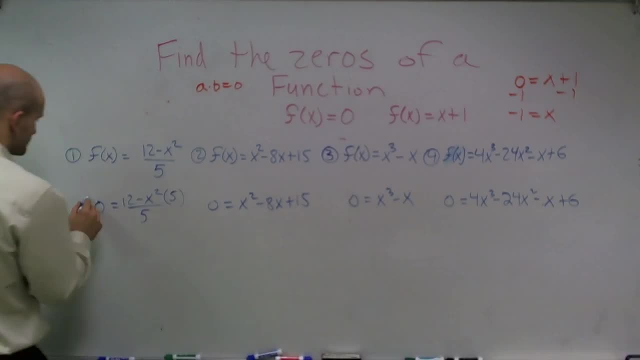 So to do that, I'm going to multiply by 5 on both sides. That still gives me 0.. So I have 0 equals 12 minus x squared. Well, what I can do is add the x squared to the other side. 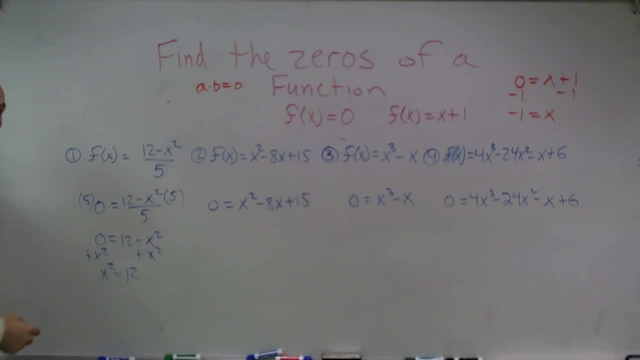 So I have x squared equals 12.. Now, remember, I'm going to have to take the root of both sides. so x is going to equal plus or minus radical 12.. Now I can simplify radical 12 into 2, radical 3.. 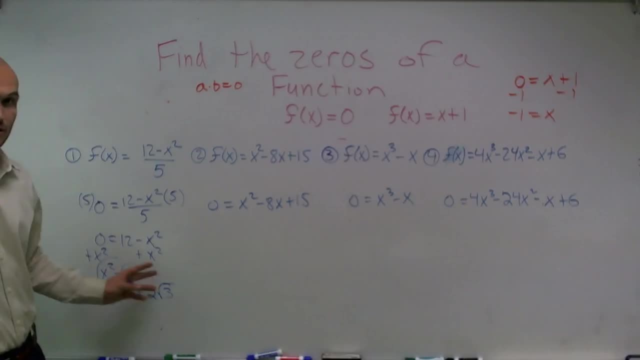 But remember just, whenever you take the square root of both sides, it's going to be plus or minus, For here I have an x squared minus 8x plus 15.. So therefore, I'm going to have to look into some kind of factoring. 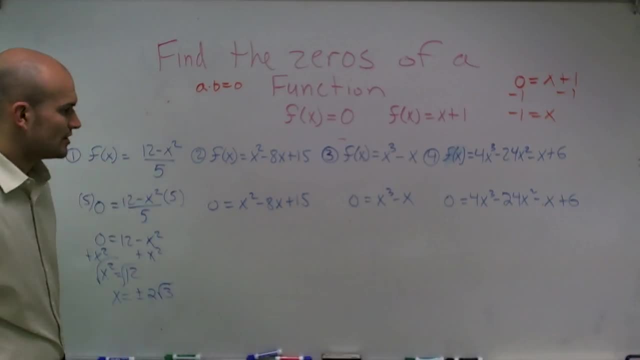 I just can't add these over and solve for x. I have to factor this. So I look at what two numbers multiply to give me 15, but add to give me negative 8? Well, I say 0 equals x minus 3.. 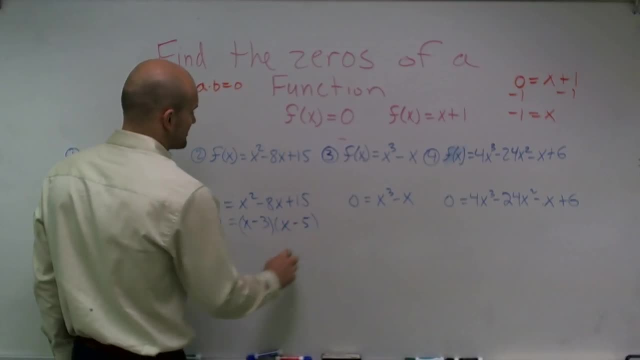 And x minus 5.. Because negative 3 times negative 5 is positive 15.. Negative 3 plus negative 5 is equal to negative 8. So therefore now, since both of these multiply by each other equals 0, I can set them both equal to 0. 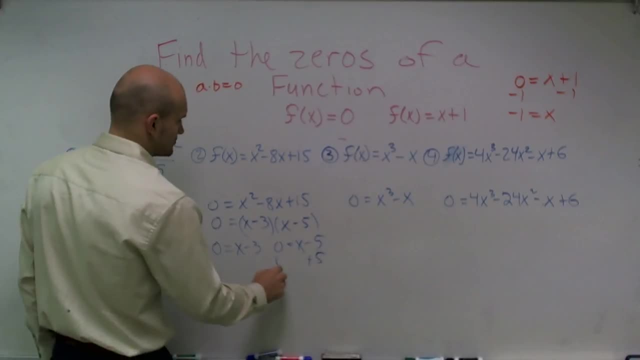 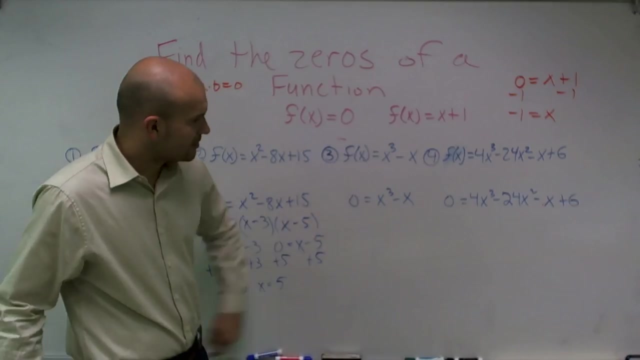 Now solving for x, I get x equals 3, and x equals 5 are my two 0's. This one is a little bit more difficult. Well, because here you know what do I do? I add the x over to the other side. 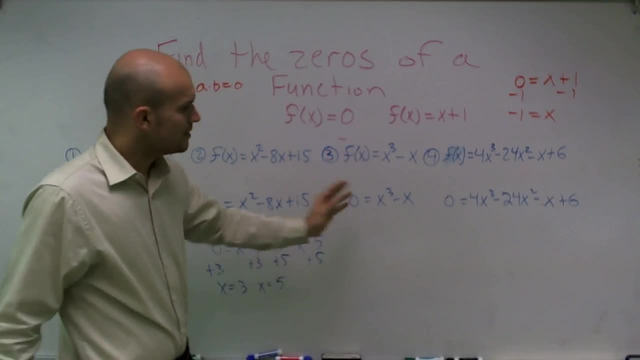 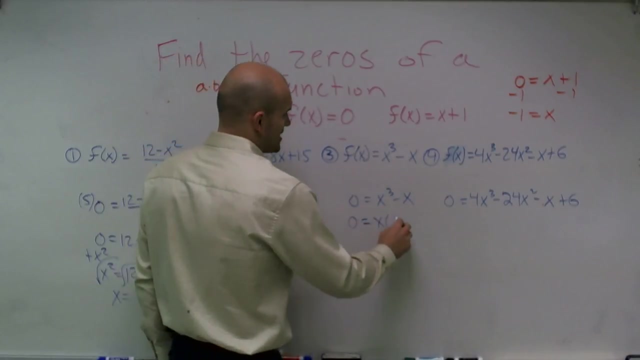 root it by 3.. I mean, what am I doing here? Well, remember, always try to see what you can take out of each function. So I can factor out: an x 0 equals x times x squared minus 1.. 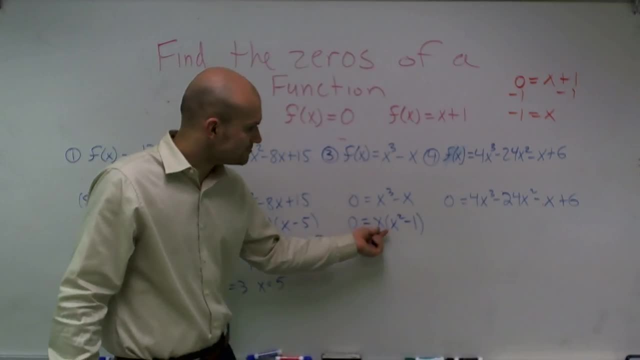 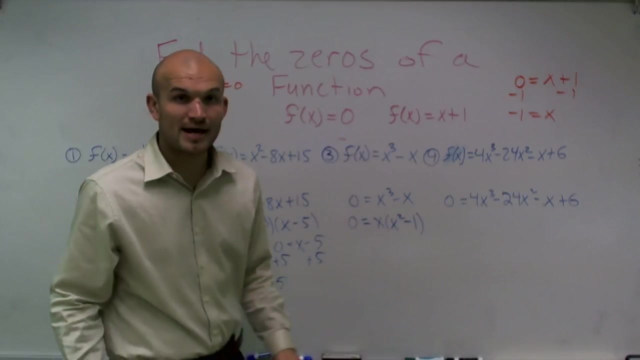 So now here I have now a term, a term multiplied by another term. So therefore, or not, a term, but a binomial multiplied by a binomial. So then what happens is, again I can use my 0 product property. 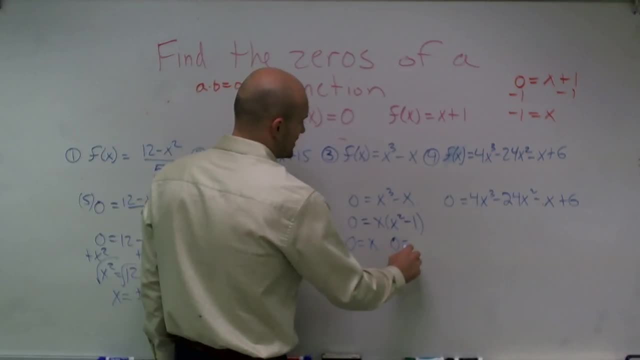 So I can say 0 equals x and 0 equals x squared minus 1.. Now, solving for x, I get 0 equals x and x squared equals 1.. Take the root of both sides: x equals plus or minus 1.. 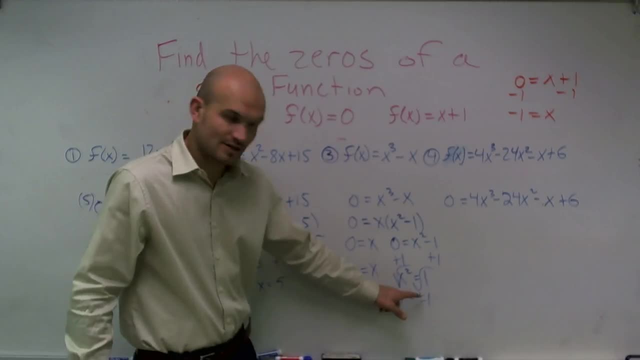 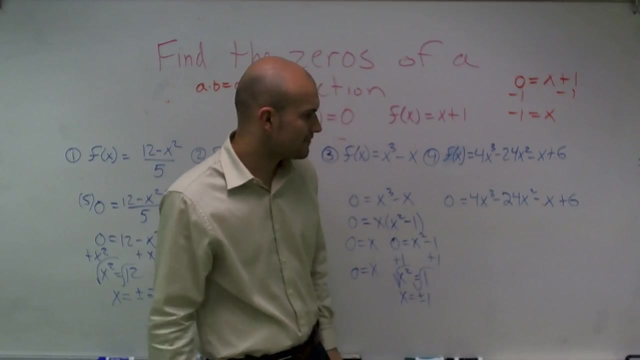 Therefore my 0s are x equals 0, and x equals plus or minus 1.. For the final problem, again, I have factoring by grouping. So what I'm going to have to do for here is group the first two terms. 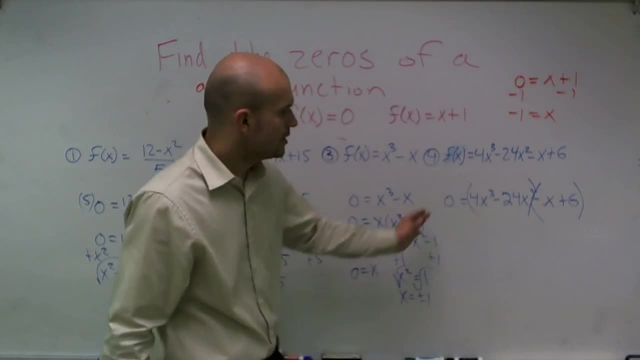 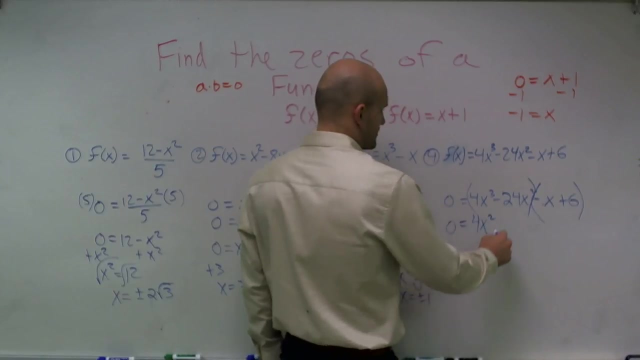 and group the last two terms. Now see, what can I take out of my first two terms? Well, to factor out my first two terms, I can take out a 4x squared And that's going to leave me with, actually, you know what. 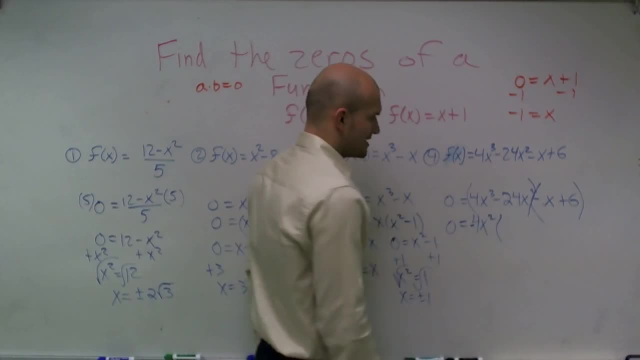 To make this look like that one, let's take out a negative 4x squared, Because if I take out a negative 4x squared, I'm going to be left with a negative x plus 6. And then here I can't. 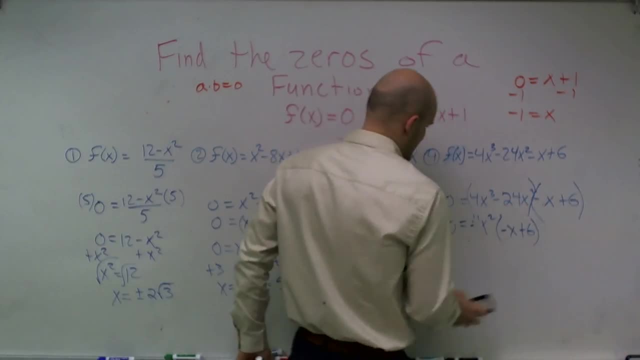 actually. well, that'll make sense, That'll work with that one. Well, yeah, let's just leave it like that. And then this will be times a negative x plus 6.. So if I was going to, I'm sorry, plus. 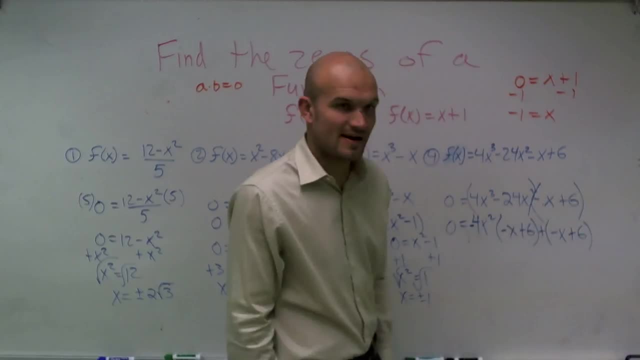 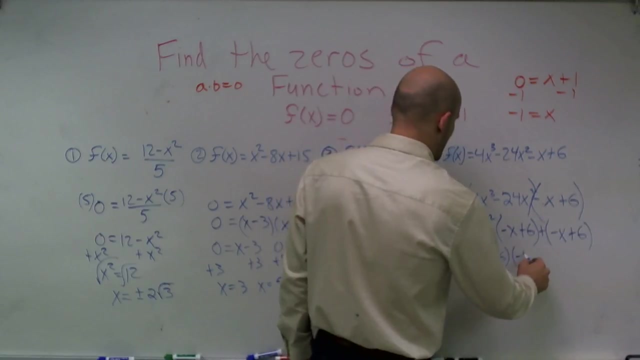 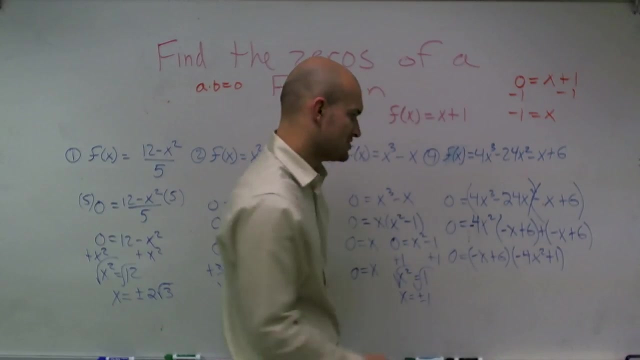 so now, if I'm going to factor out a negative x plus 6, I'll be left with a negative x plus 6 times a negative 4x squared plus 1. Because, remember, there's a 1 times that factor. So now to solve each of these equal to 0,. 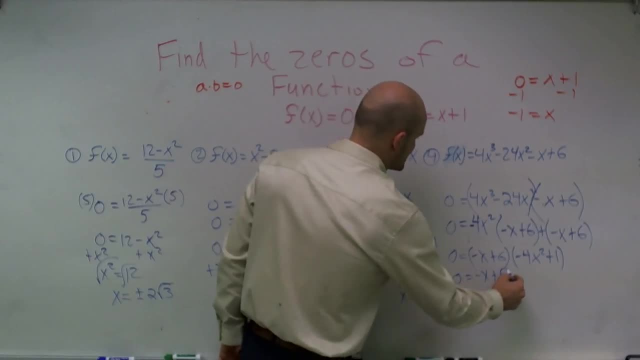 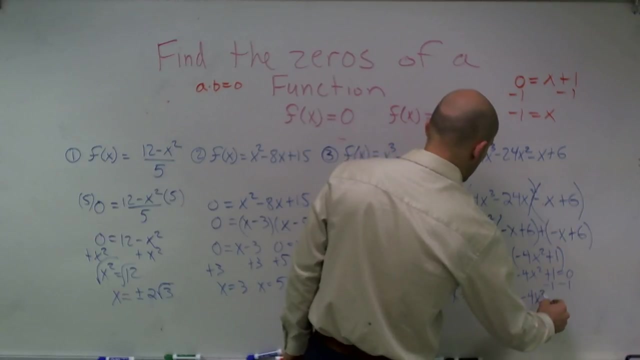 I have: 0 equals negative x plus 6 and negative 4x squared plus 1 equals 0. So therefore, x equals 6 is 1, 0. And here I need to subtract 1,, divide by negative 4,. 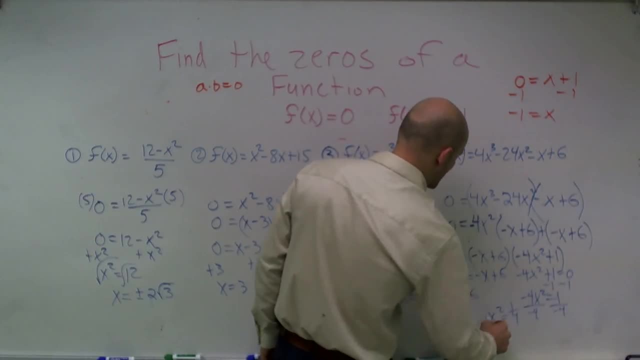 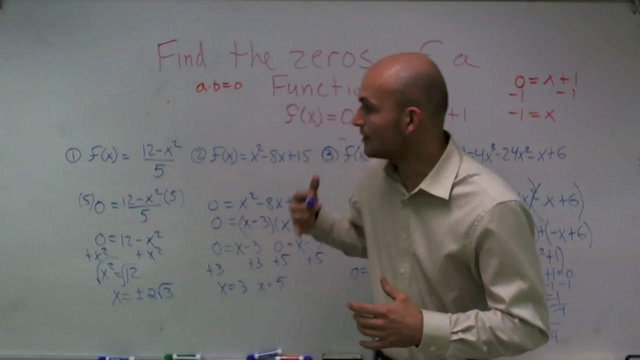 and say: x, squared, equals 1 fourth. Take the root, Oh man, And I get: x equals plus or minus the square root of 1 fourth. All right guys, That's how you find the zeros of a polynomial function. I hope this helped you out. 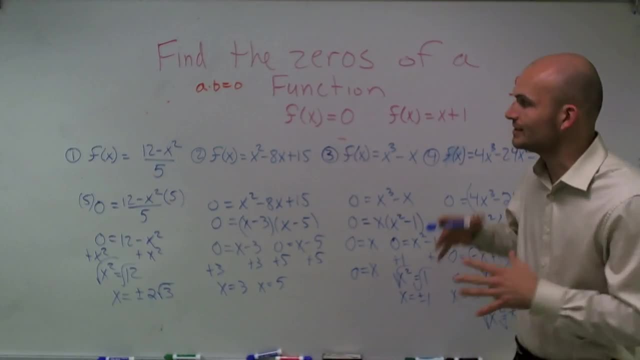 Just a couple tenements. Just make sure you remember your rules are for solving And just remember, whenever you're trying to find the zeros, just take your f of x equal to 0 and find the values of x that make it 0..